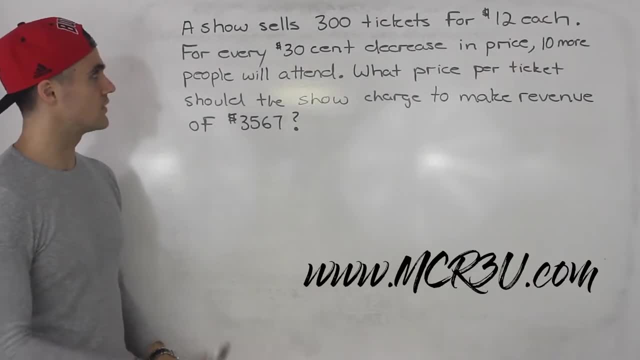 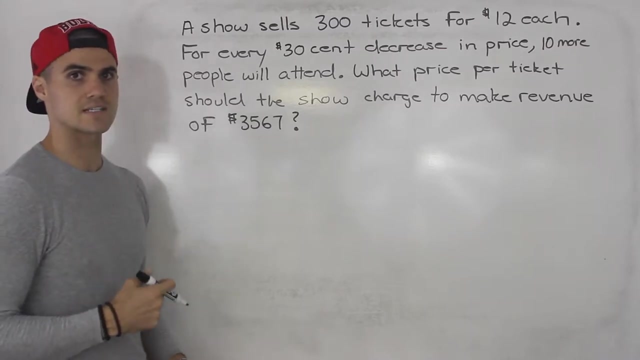 Welcome back everybody. Moving on with quadratic equations, We're told that a show sells 300 tickets for $12 each. For every 30 cent decrease in price, 10 more people will attend. What price per ticket should the show charge to make revenue of $3,567?? So this type of question we have to. 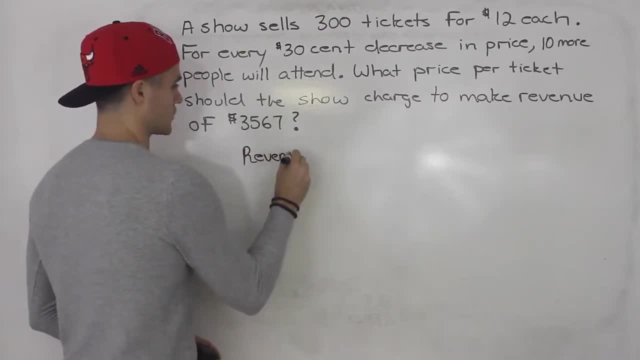 make a revenue function And we know revenue is equal to what Price per item times the number of items. In this case we're dealing with tickets, so the number of tickets. But this is the general formula. Price actually let's write per item times number of items. So currently, 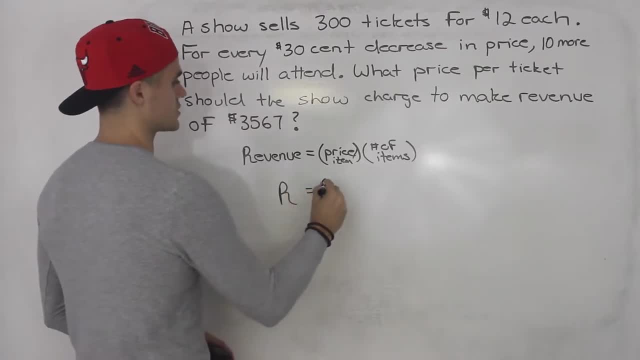 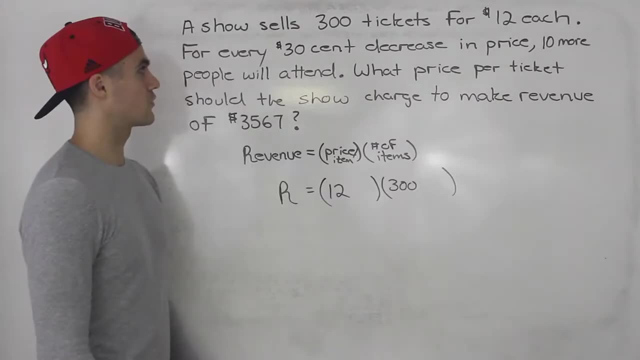 the price per ticket is $3,567. And we know revenue is equal to what Price per item times per ticket is $12.. And the number of tickets being sold is 300.. Now we're further told that for every 30 cent decrease in price, 10 more people will attend. So let's introduce a variable. 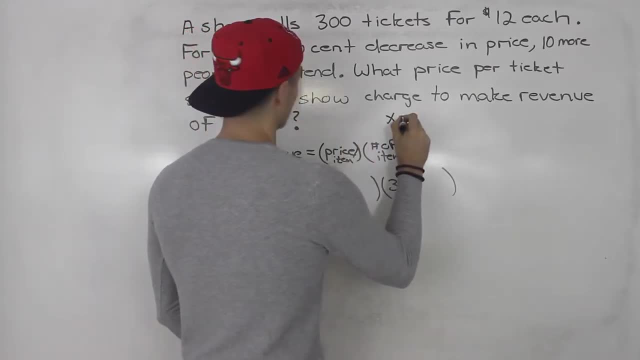 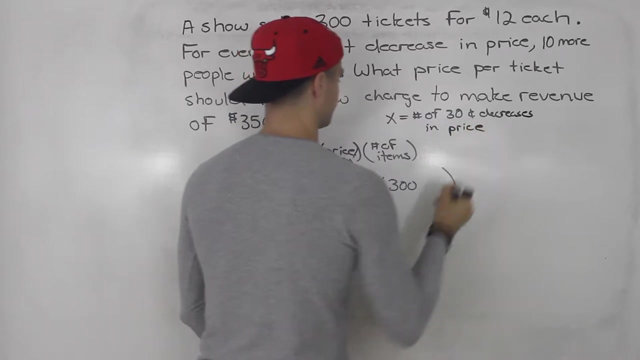 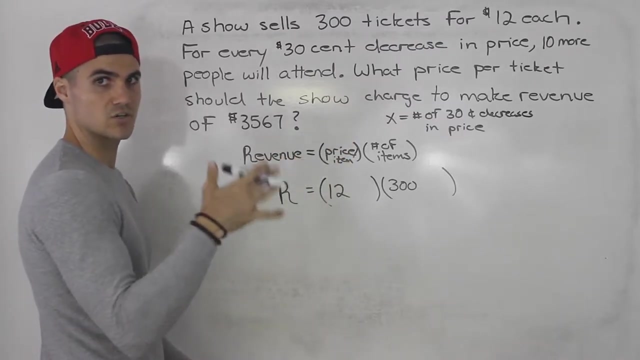 here. Let's say we let x equal. the number of 30 cent decreases And we're decreasing the price x number of times by 30 cents, or $0.3.. And for every 30 cent decrease in price, 10 more people will attend. So this would be plus. So here's $13.. So let's say we let 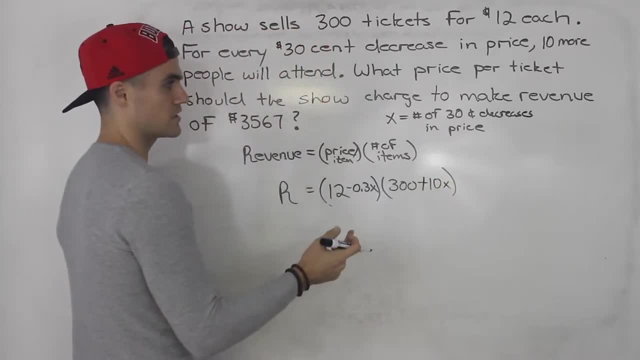 10x. So if we decrease the price by 60 cents, so x would be 2,, then 20 more people are going to 10, 20 times 2, and so on and so on. So this here is your revenue function, And they are asking us. 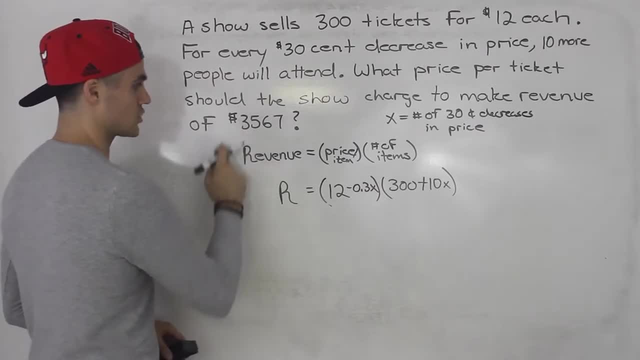 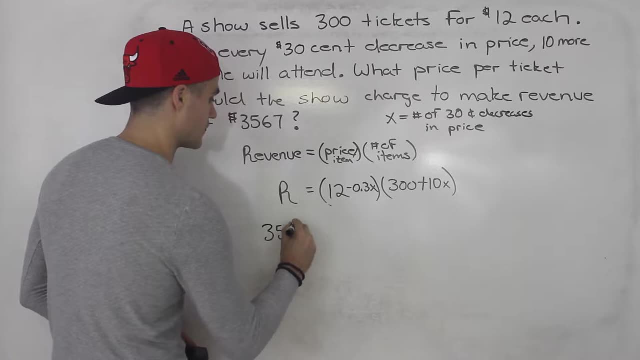 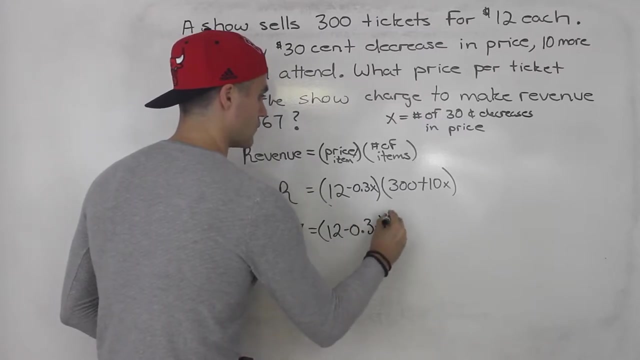 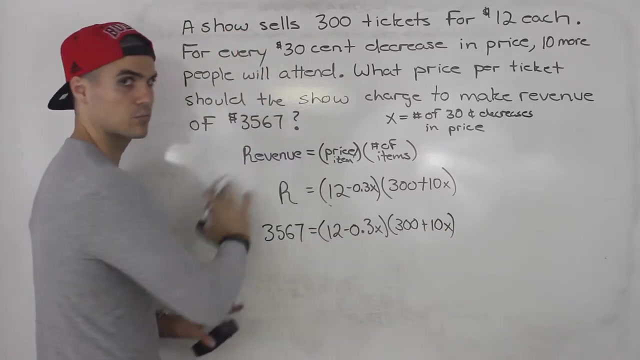 what price per ticket should be charged in order to get a revenue of 3,567.. So what we would do is we would plug in 3,567 for the revenue And then we can just solve for x. This is just an equation. now We can expand everything, bring it over to one side. 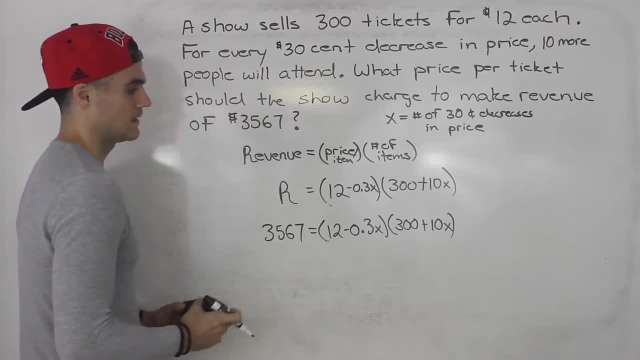 either factor or use the quadratic formula. Now, one thing I want to mention is this question is similar to other revenue questions we've done, But usually what they've been asking us before is to find the maximum revenue, So we're not plugging in. 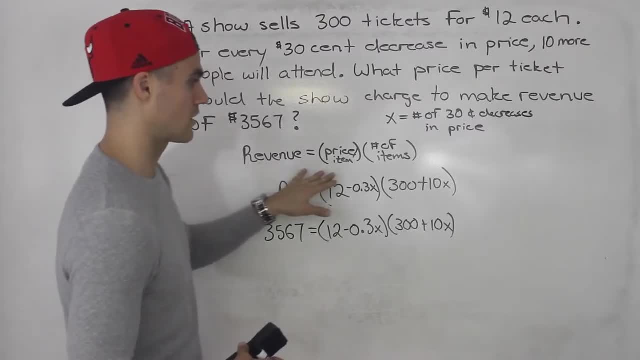 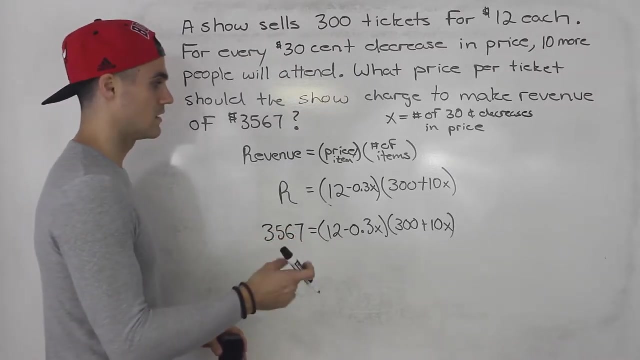 anything for r. in those cases We are expanding this and completing the square. Or you can find the intercepts and then find that max vertex that way as well. So basically, in those questions when they're asking you for the maximum revenue, they're asking for the vertex of this function. 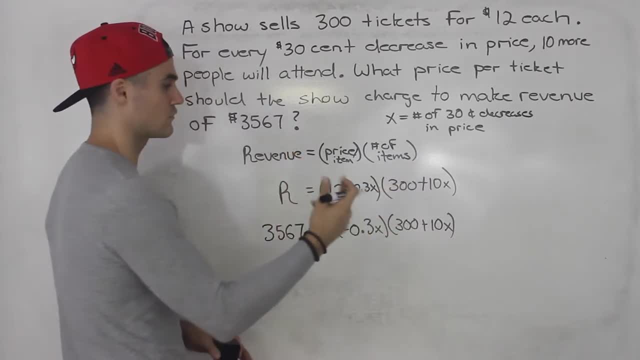 They're asking for the ticket price or the number of items. you plug in that x value of the vertex in these brackets. But in this case they're giving us a specific revenue, So we have to plug that revenue in here And then we have to solve for x. We're not finding the max, we are solving for x. 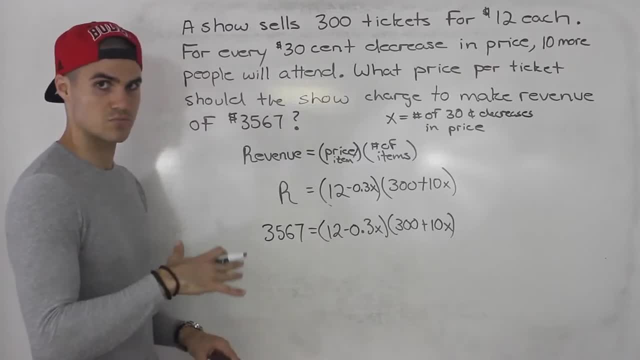 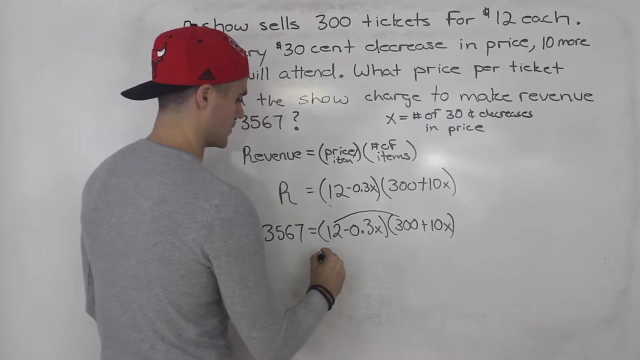 So just make a note of the differences between questions before dealing with revenue in this chapter and this question here. So to solve this now, we're just simply going to expand this. bring this over: We'll have 12 times 300, which is 3,600.. 12 times 10x gives us 120x Negative, 0.3x times 300,. 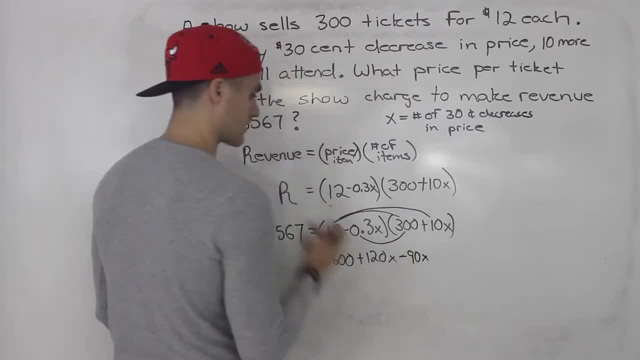 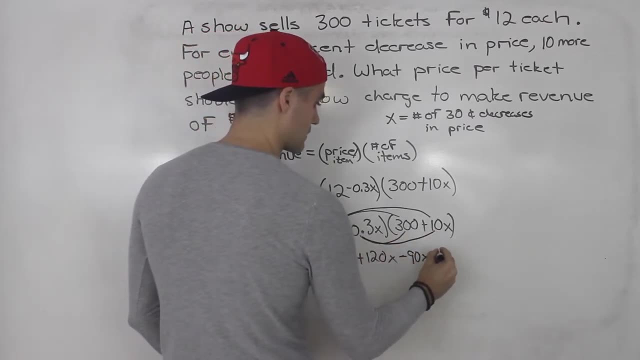 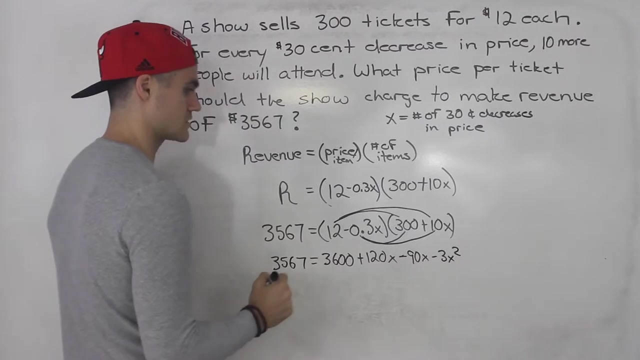 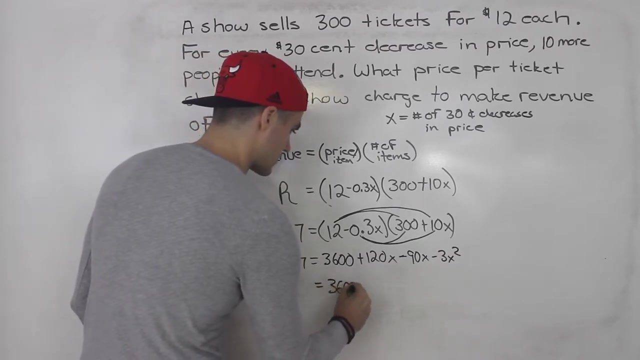 that gives us negative 90x, And then negative 0.3x times 10x gives us negative 3x squared And 3,560.. 3,560 is on the left side, So here we'll have 3,600.. This would be 30x. This would be minus. 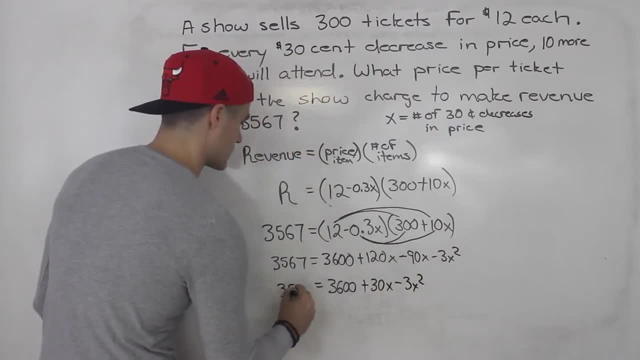 3x squared, This 3,567 is still here. Let's actually bring everything over to the left side just because this is a negative 3x squared And I always like to usually have the leading coefficient be positive, But either way works. 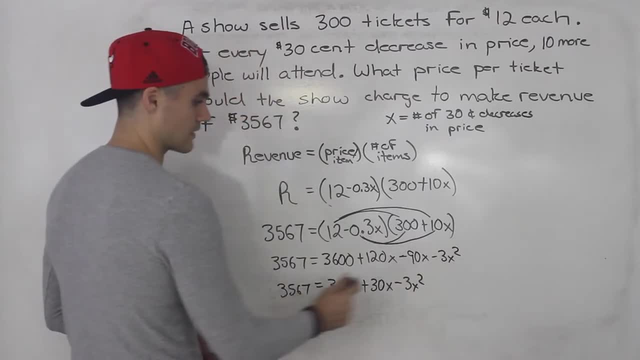 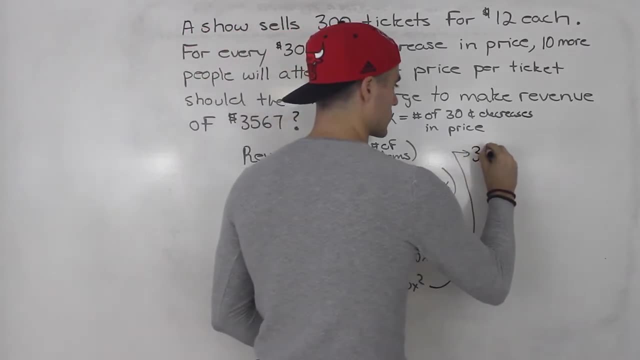 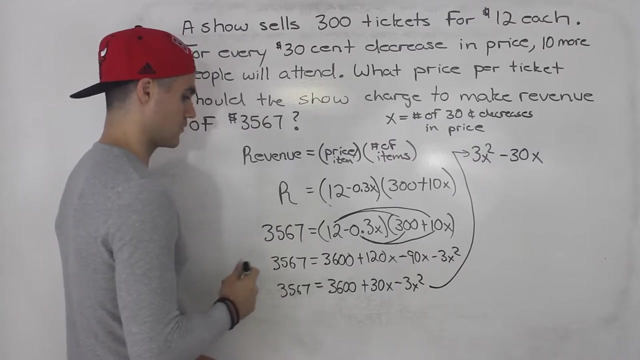 But yeah, personally I'm going to bring everything over to the left side. So, continuing this up here, this would come over, So it'd be 3x squared positive, 3x squared. This 30x would come over, So that would be minus 30x, And then 3,567 minus 3,600.. That would give us negative 33.. 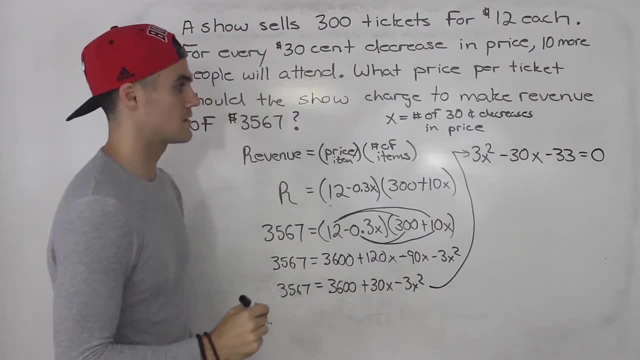 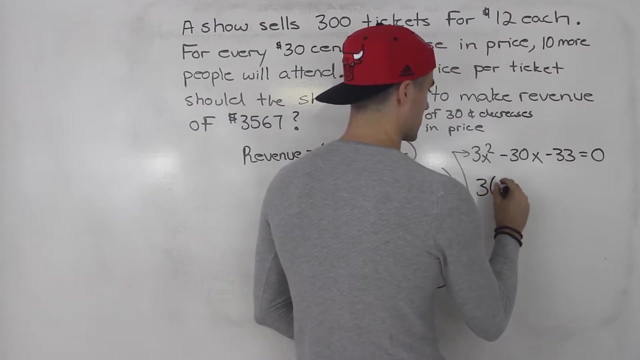 And that would equal zero. There would be nothing left on that right side. So we have a quadratic equation here. You can throw that into the quadratic formula if you like. I think this is actually going to factor smoothly. So let's take out a 3.. So we would have: 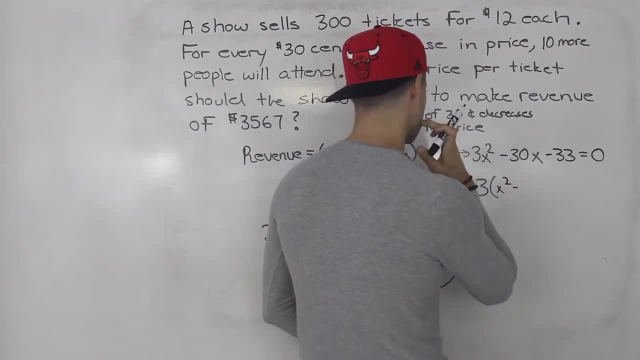 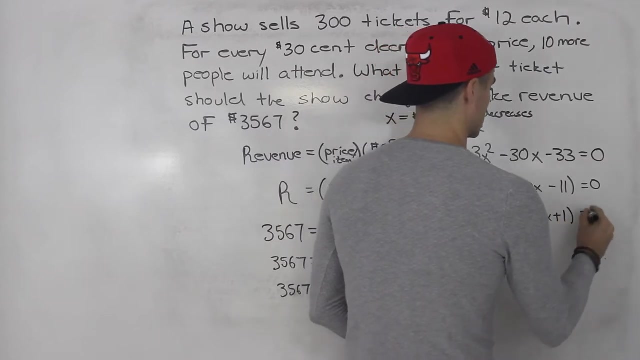 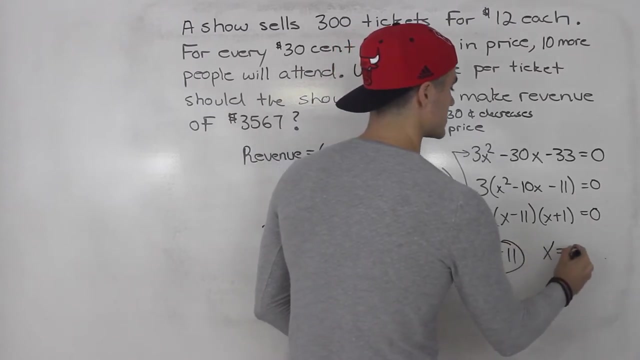 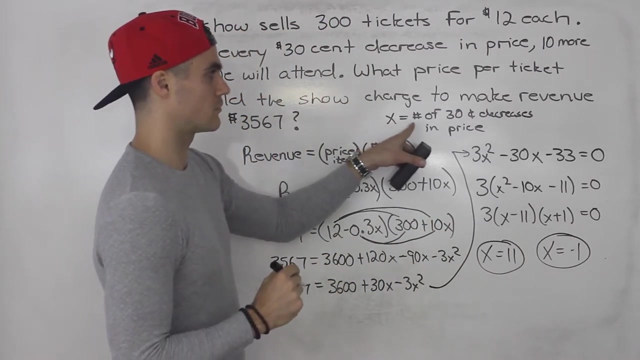 x squared minus 10x minus 11.. So 3, this would be x minus 11.. This would be: x plus 1 equals 0. Then, from here, x is 11 or x is negative 1.. And what does x represent? Well, x represents the number of 30 cent decreases in. 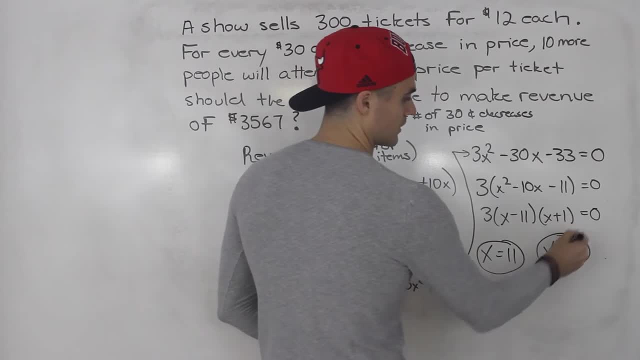 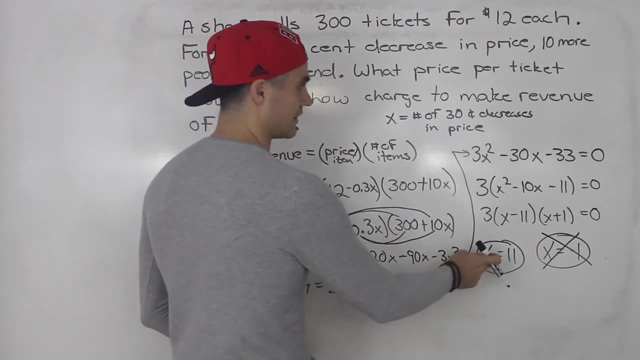 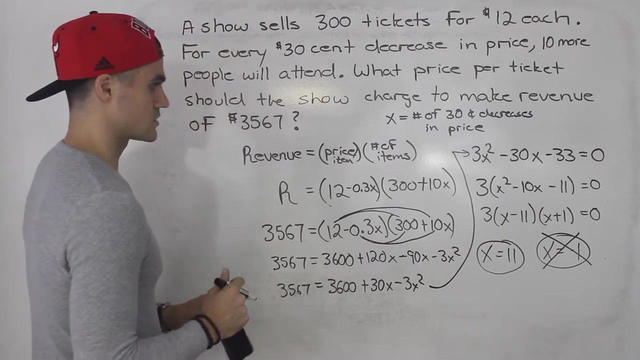 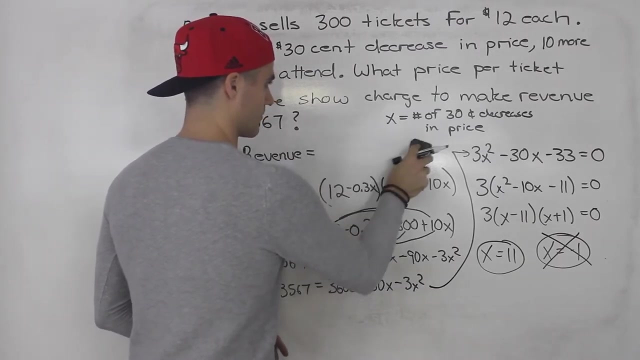 price. So notice this: x value negative 1, we would ignore. x has to be positive always. So we're going to have 11- 30 cent decreases in price in order to get this revenue of 3,567.. So I'm going to erase this here Question is asking us: what price per ticket? 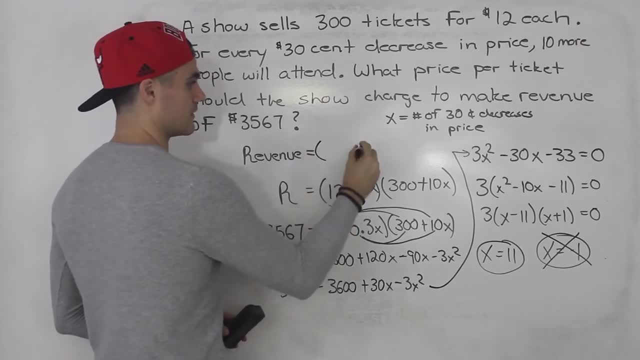 should the show charge, And this bracket is the price per ticket. So we would plug in this x value of 11 into this bracket. So 12 minus 0.3 times 11.. That's like 12 minus $3.30,, which is $8.70.. So that's the price per ticket that should be charged. 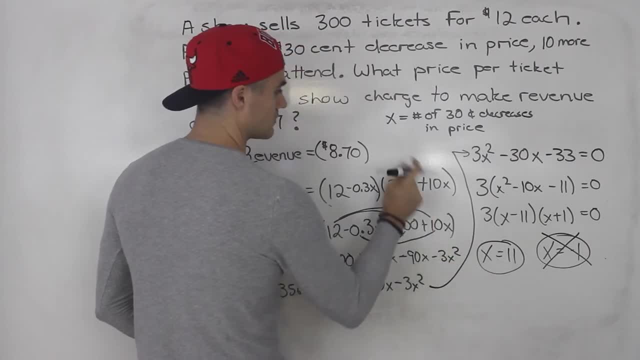 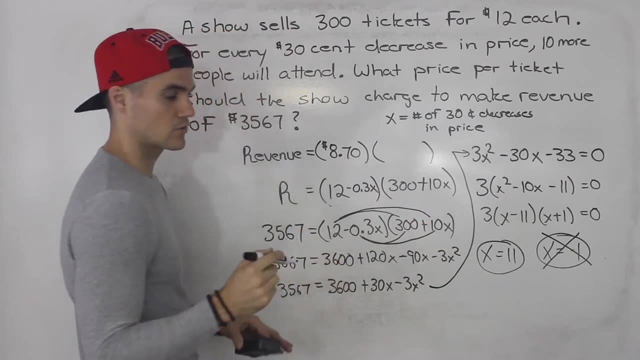 And then, to check your answer, you could plug in this x value of 11 here. That's the number of tickets that are going to be charged. So that's the price per ticket that should be charged And the price per ticket that's going to be sold. so 300 plus 10 times 11 is 300 plus 110,.